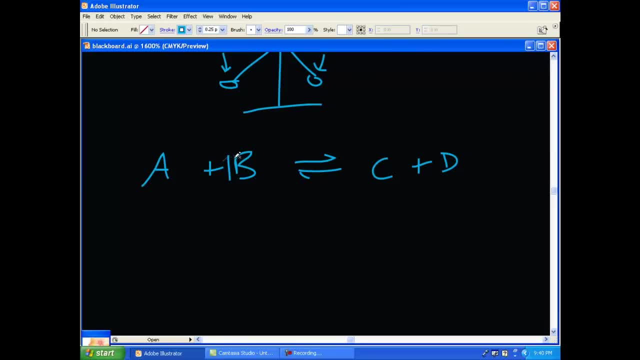 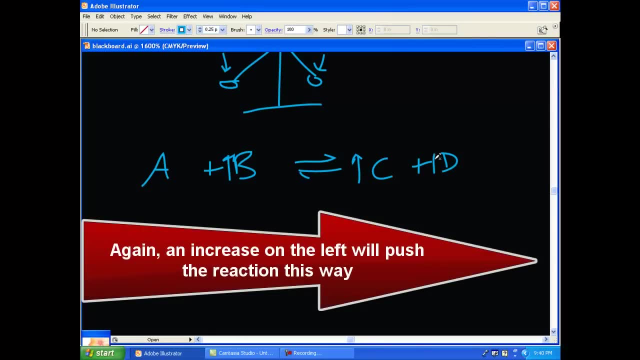 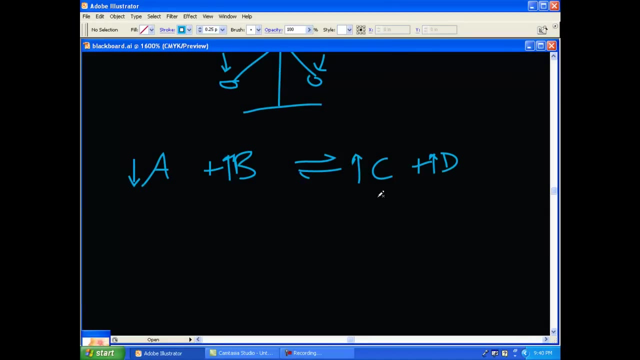 And now, instead of increasing A, you increase B. Well, again, increase the left side. So what does nature do? Well, it increases what's on the right And you're going to eat up some of the A. So if you increase B, it's going to push the reaction. 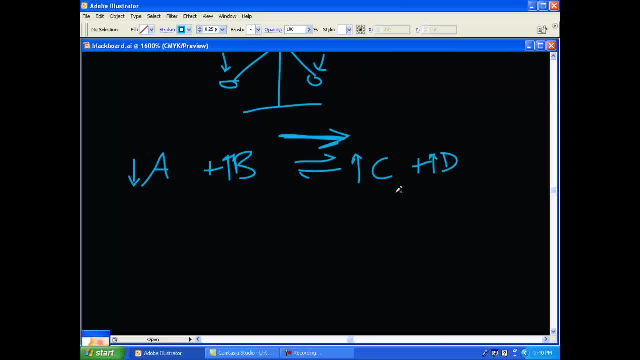 This way, so that now you have more C and D, since you're adding more reactant to it. So let's see what happens when we increase one of the products. If we increase D, well, what's going to happen to the left side? 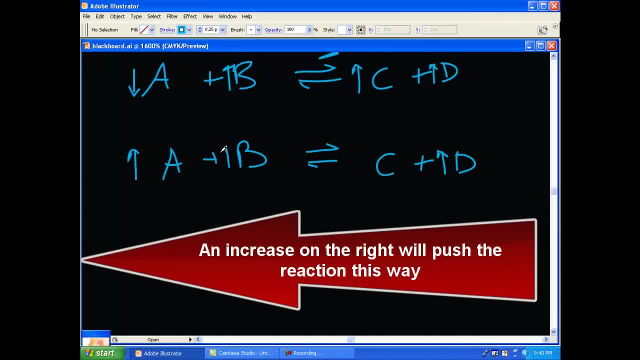 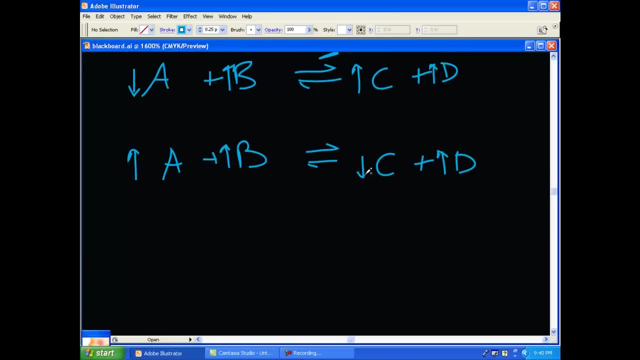 Yeah, we're going to have to increase it right, Balance it out And you're going to get some a little bit less D to also make up for the increase in, Or less C, rather, to make up for the increase in D. 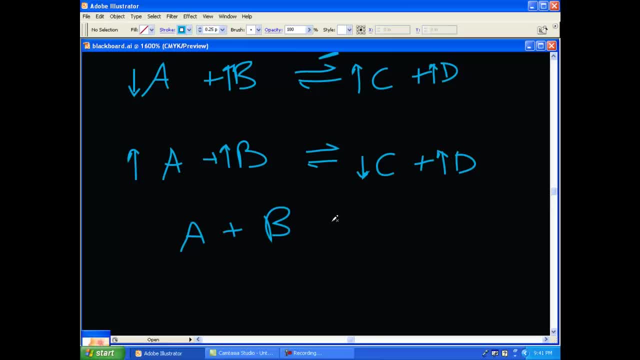 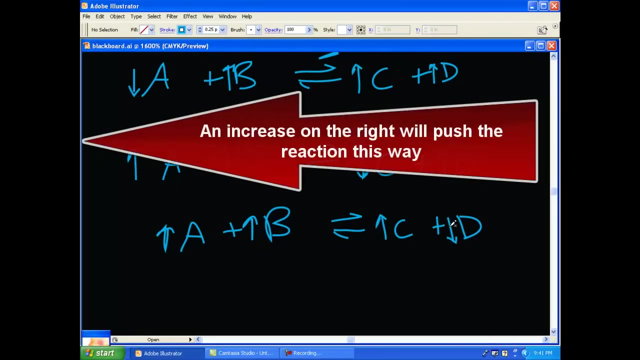 And let's say you had, After the reaction, come to equilibrium. We have an increase in C. Well, increase the right. Yeah, we're going to have to increase the left too, And D is going to slightly increase. If we increased D also, we would just get more of an increase in A and B. 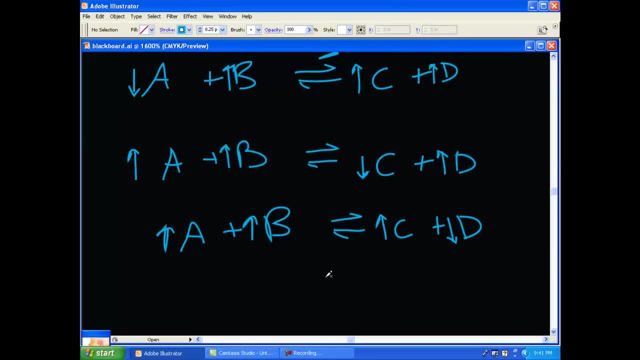 Right. So it depends on what you're adding to it. It's definitely going to affect the other side in the same way, And the more you add, the more it's going to push the reaction. right Now, let's say: instead of adding something, we take away A. 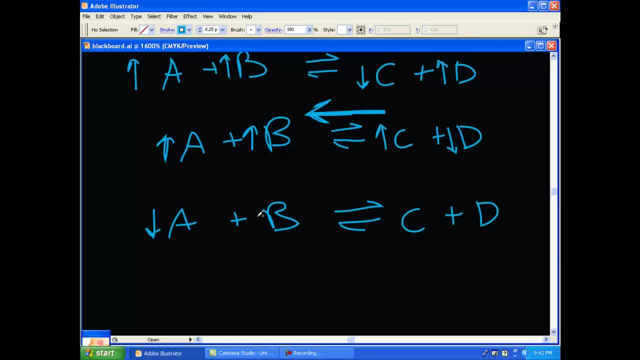 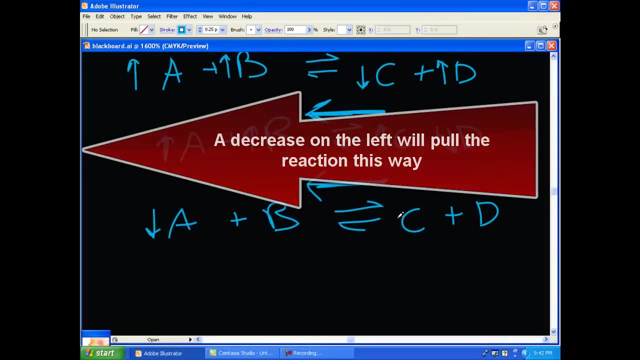 So we lower A. Now it's not. The reaction is not going to be pushed towards the right anymore, It's going to be pulled towards the left. So we're taking something away. Okay, more C and D is going to react. 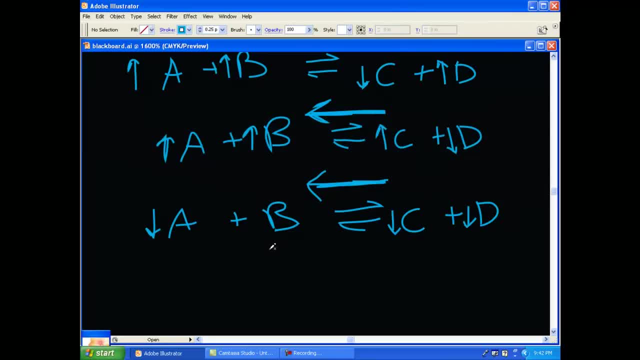 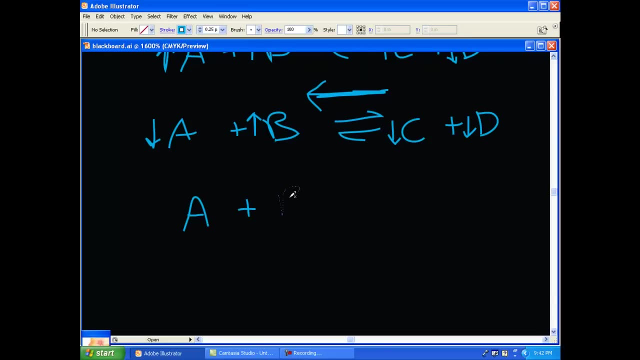 So this is going to decrease as well. on the right, And we're going to get an increase in B, Since more C and D are acting together, but we're taking the A away right And in a similar case, if we have 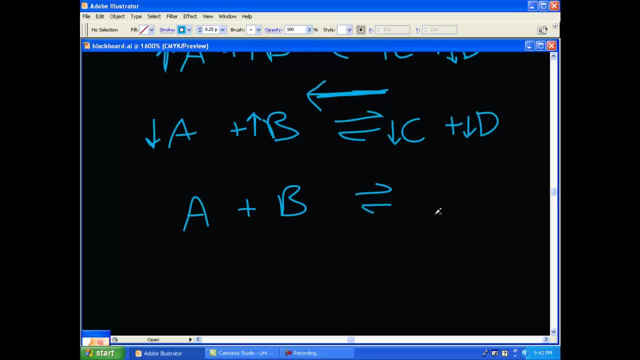 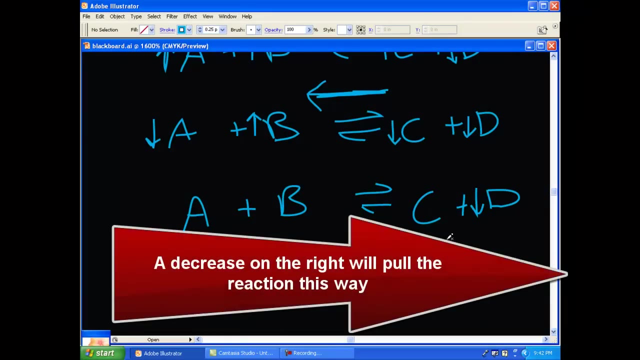 I'll just randomly take away one of the products after the server reacted. For example, let's say we take away D. Well, if we take away something, we're going to get an increase in B. So if we take away something on the right now, the reaction is not going to be pushed anymore. 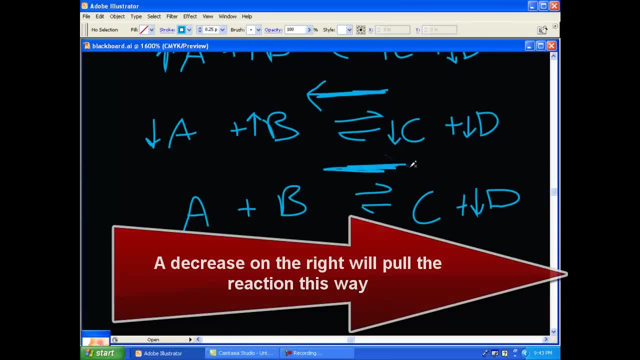 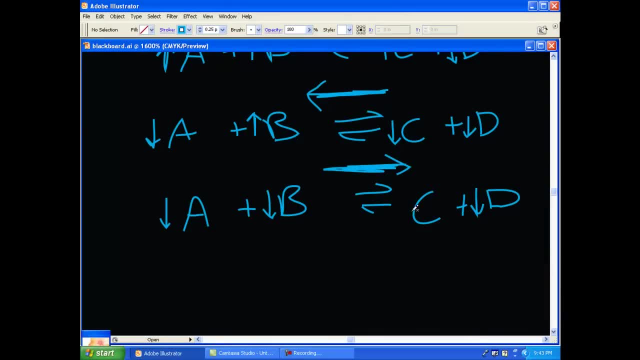 Again, it's going to be pulled into this direction, so that more A and B are reacting, And it's going to result in a decrease in A and B With an increase in C, since we're not removing the C, we're only removing the D. 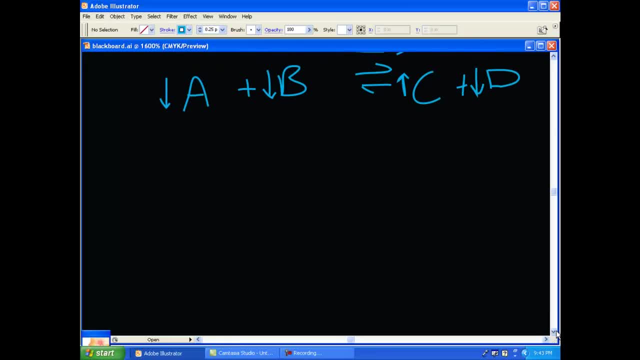 Okay, So those are the different scenarios you can have. A reaction is either going to be pushed in one direction. if you're adding it to one side, It's going to be pushed to the other direction. If you're taking something away, either a reactant or a product, it's then going to be pulled in that direction. 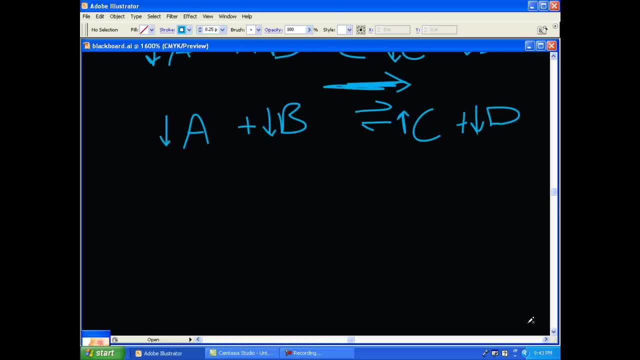 Whichever one you're decreasing. Okay. So what if you had An endothermic reaction, where heat needs to be added to one side in order for the reaction to take place and you take away the heat? Well again, if you lower the heat, you're not going to get as much A and B forming together to make C and D. 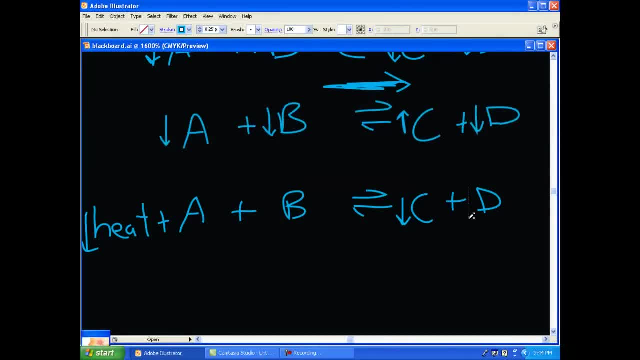 Or reacting together, rather to form C and D, And C and D is going to decrease. Okay, A and B is going to increase Because you're taking away that heat for them to react together. Alright, Now let's say you had. 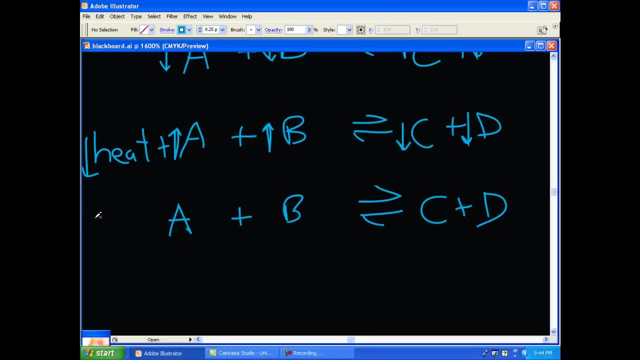 An endothermic reaction Which again thrives on heat Right, And you added more heat to it. Well, if you add more heat to it, you're going to have a greater reaction of A and B. So the concentration of A and B separately is going to come down to increase more C and D. 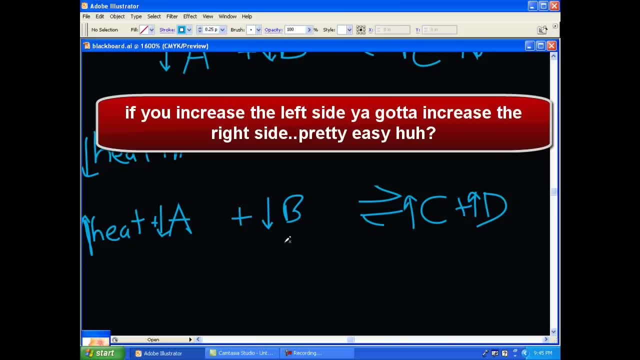 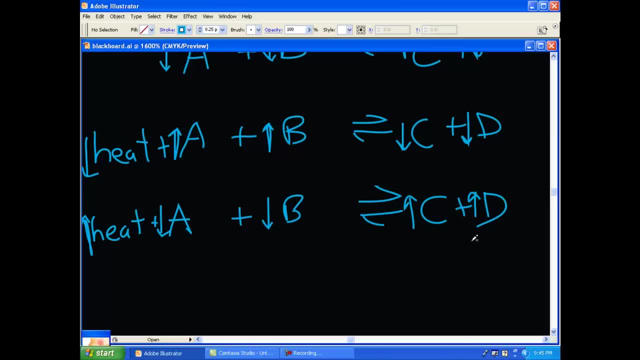 Right, Like if you add extra heat to fry, let's say, fry an egg, Right, You're going to get less of the original and more of the fried egg To products. Okay, Now if you add A plus B again, 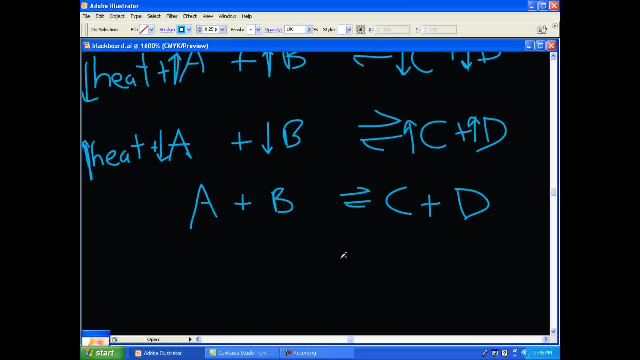 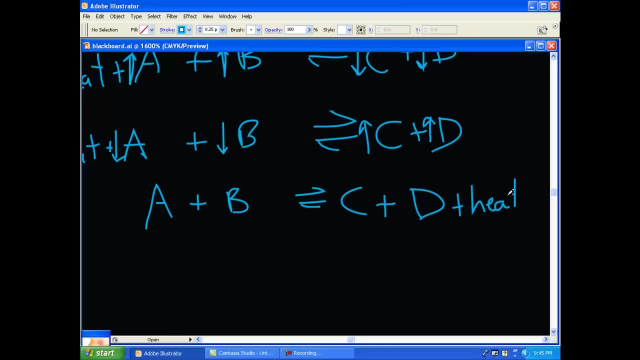 to your C plus D, and now you don't have an endothermic reaction. you have an exothermic reaction, Which means that heat is being released as C and D's, your products are being produced And you cool down the entire system. 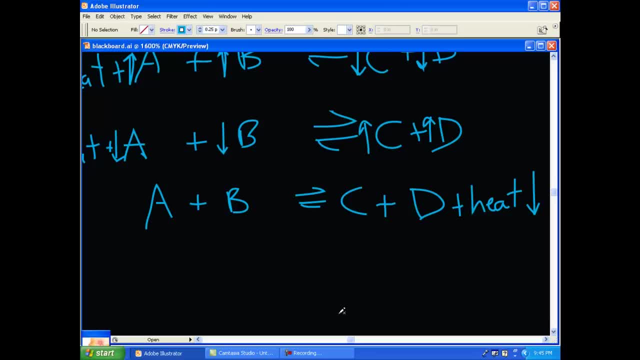 so you lower the heat. well, if you lower the heat or take it away, you're gonna be pulling the reaction in this direction, right. so you're gonna have to lower what's on the left side to balance it out. you're gonna have an increase in C. 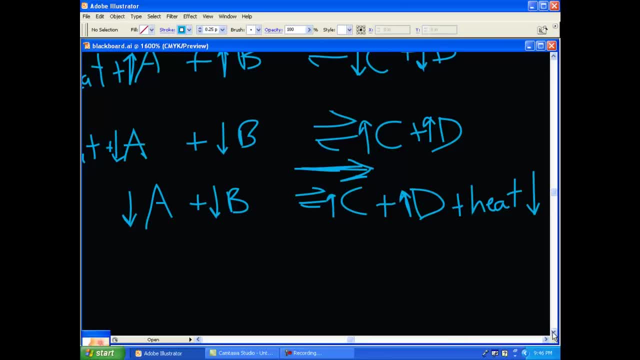 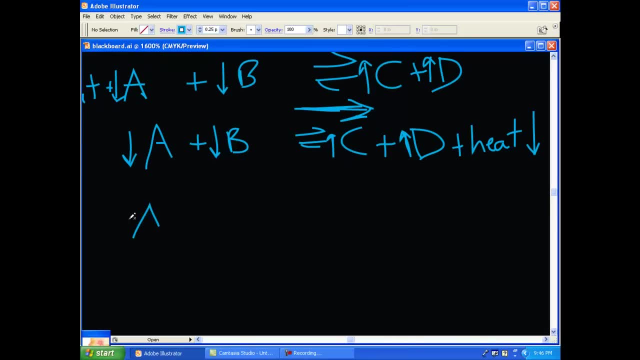 and D and, let's say, the final scenario you could have is a plus B. you'll C plus D, again in an exothermic reaction that yields heat, and now you add more heat to the system. well, if you add more heat to the system, what's gonna happen? well, yeah, 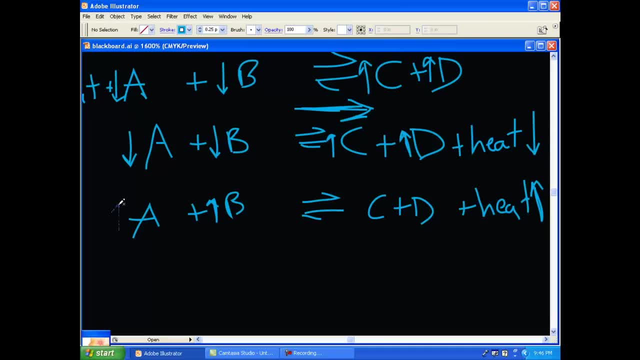 you got you increase the right, you got to increase the left. so what's going to push it in that direction? and you're gonna have a decrease in C and D. so those are all the different scenarios on how concentration and temperature can affect the system that's at equilibrium. if you're adding something to it, it's gonna push it to. 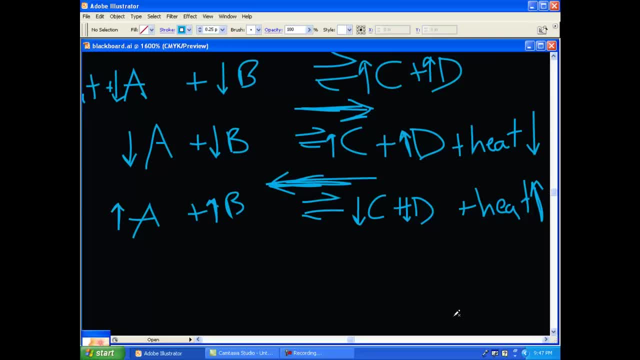 one direction or two to the opposite direction. you're gonna increase the right, you gotta increase the left, so what's gonna push it in that direction? and you're gonna have a decrease in C and D. so those, And if you take something away, it's going to pull it in that direction. 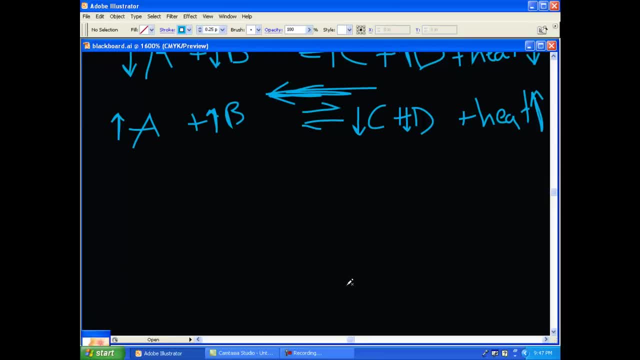 So that's pretty much it. So let's say we had N2 plus 3H2 yields 2NH3 plus 92 kilojoules per mole Exothermic reaction. right Now, if we add nitrogen, what's going to happen? 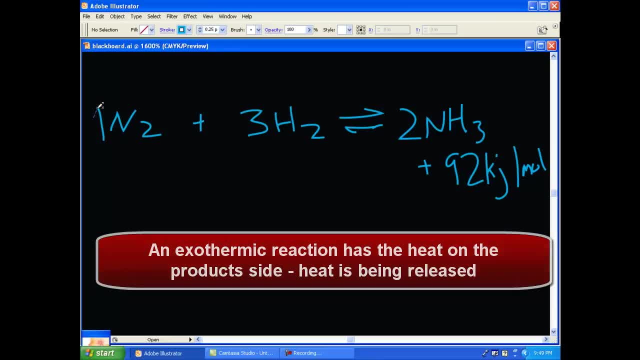 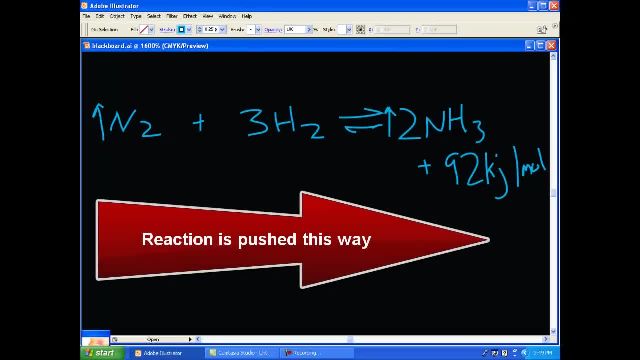 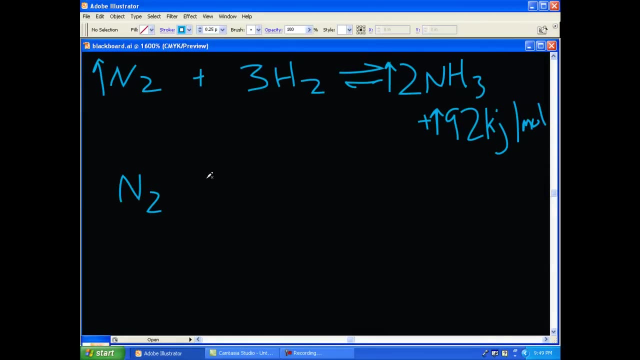 Well, if we add nitrogen to the system, we're going to get more ammonia Right And more heat. Similarly, let's say we add more hydrogen to the system, We're going to push the reaction to the right right To get more ammonia and heat. 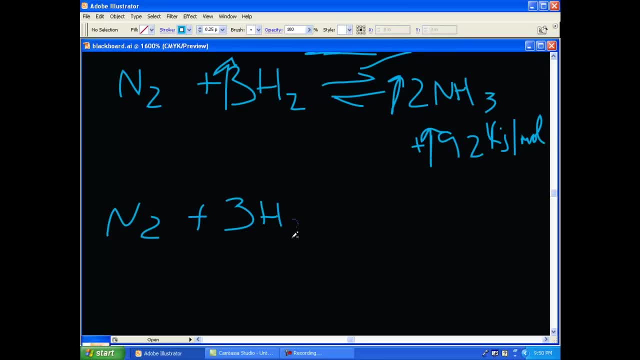 We're at it again. And now, let's say, the amount of ammonia is being decreased in this reaction. Got to write that heat in there. What's going to happen? Well, if we decrease it, it's going to be pulled in this direction. 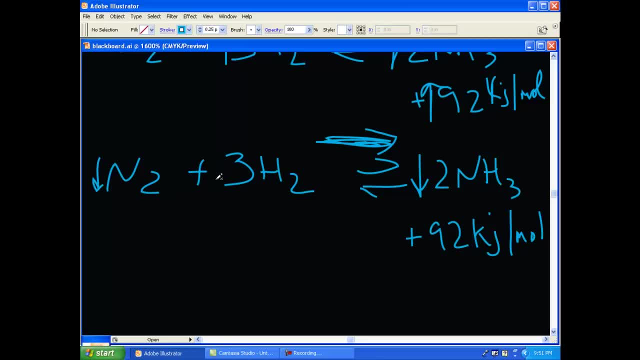 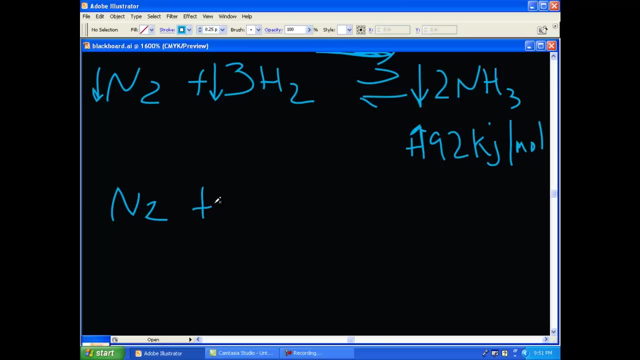 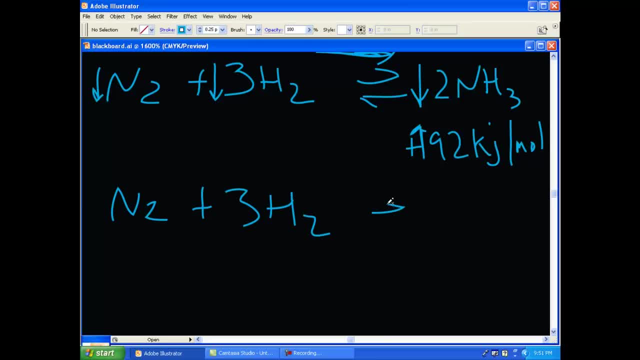